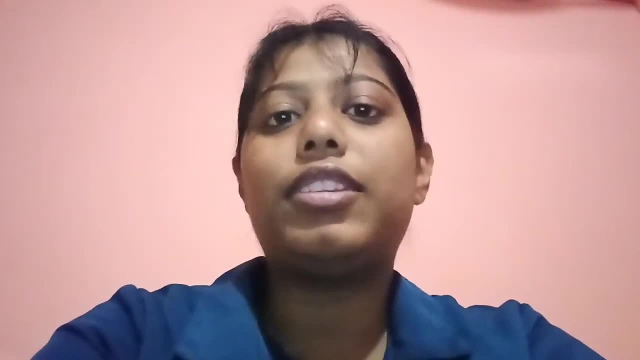 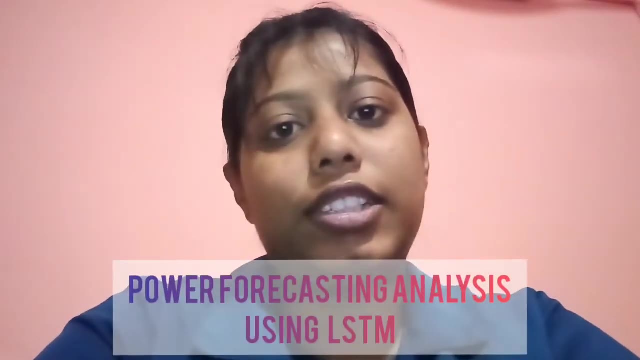 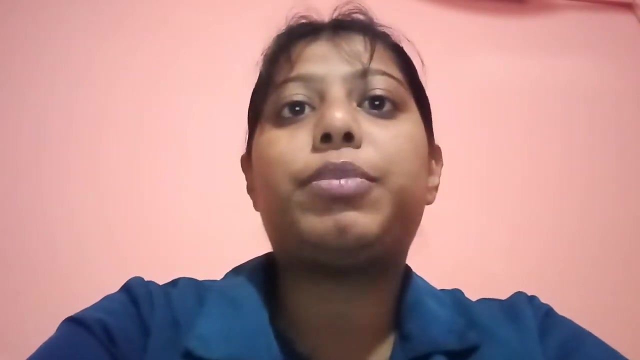 Hi, my name is Payal Das and in this video I am going to be discussing my project topic in detail. The title of my project is Power Forecasting Analysis, which we can also call as Energy Forecasting Analysis. Energy forecasting is basically a technique which predicts the future. 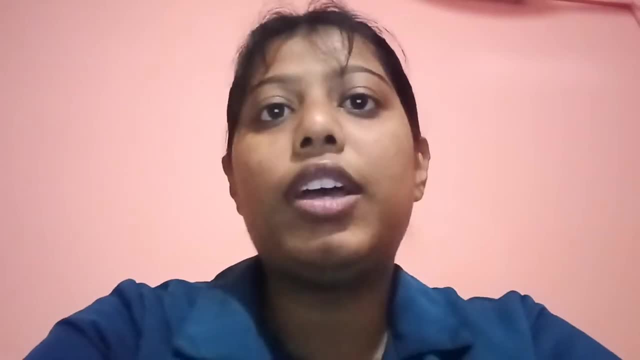 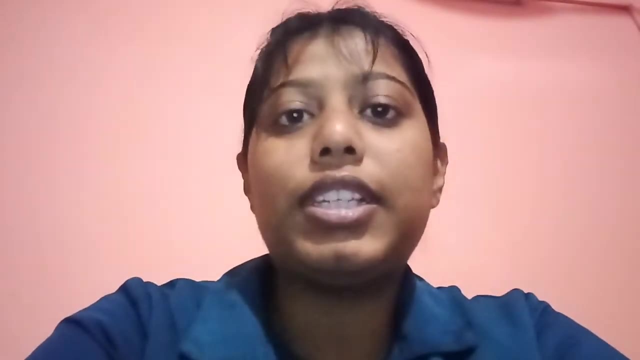 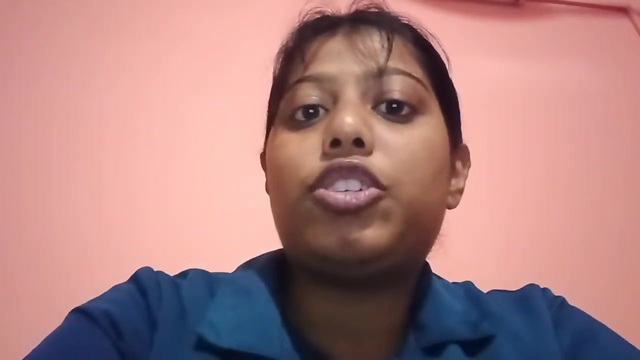 energy needs to achieve demand and supply equilibrium. The main aim of my project is to access the performance of a forecasting model, which is created using a database containing relevant information about past produced power data and data mining techniques. Let's look into the data set that I have used for this project. 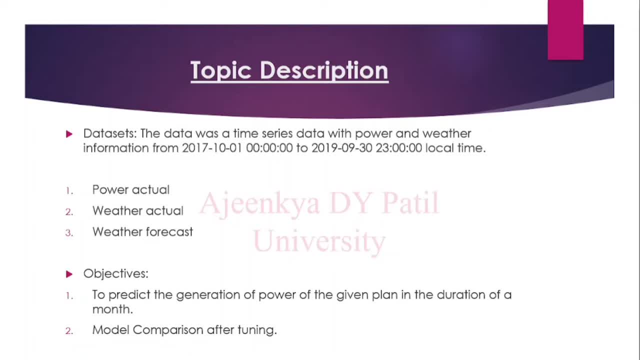 For this power forecasting project, I have used a time series data with power and weather information from year 2017 to 2019.. First data set that I have used is Power Actual, which has columns such as radiation, etc. related to solar power. Second data set is Weather Actual, which. 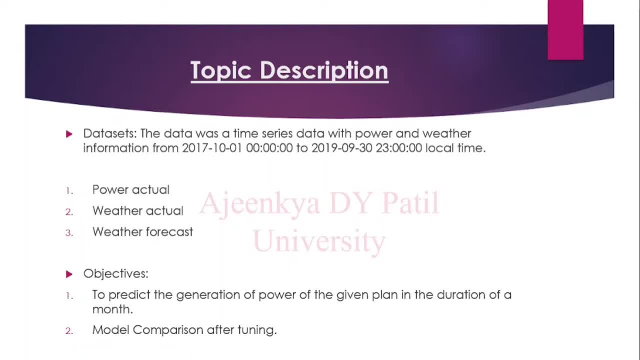 has columns such as radiation, etc. related to solar power. Second data set is Weather Actual, which has columns such as radiation, etc. related to solar power. Third one is Weather Forecast, which is basically used for testing and contains all the columns from Power Actual as well as. 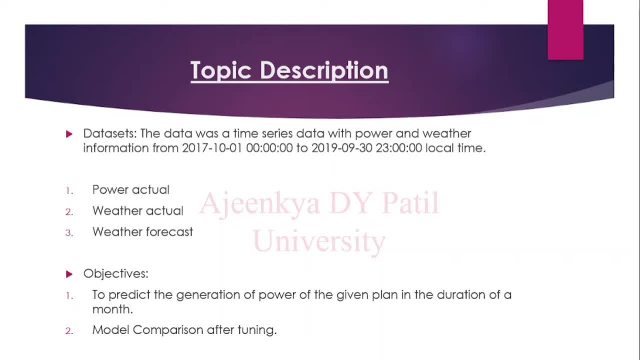 Weather Actual. The objective of our project is to predict the generation of power of the given plan in a duration of a month and then do the model comparison after hyperparameter tuning. Now let's look into our coding detail and afterwards we will also see how our project will be used in the future. 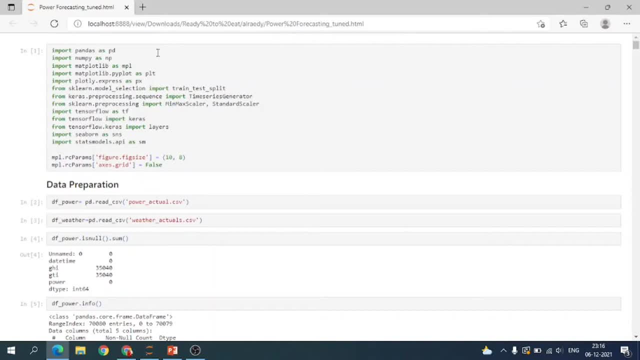 So let's look into our coding detail, and afterwards we will also see how our project will be used in the future. Okay, now let's see how this proceeded to finally get the results and outputs. Firstly, we started with data preparation and data pre-processing. 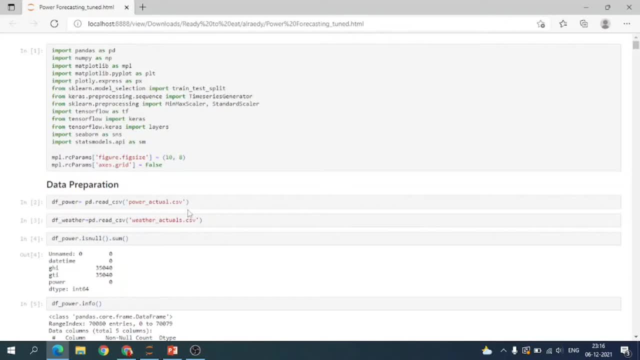 The data filed name Power Actual was having a large number of null values, and columns named GHI and GTI were having a large number of null values as well as zero. These two were basically location based data and the plant location was unknown to us at first. 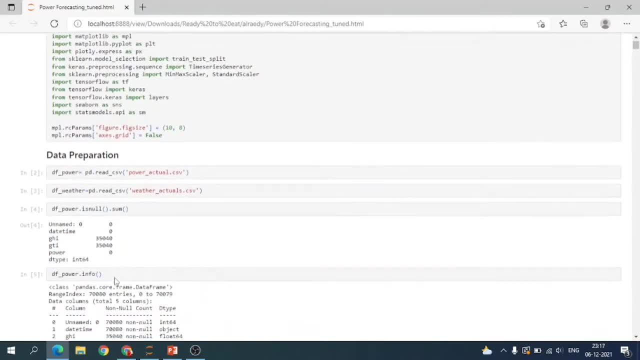 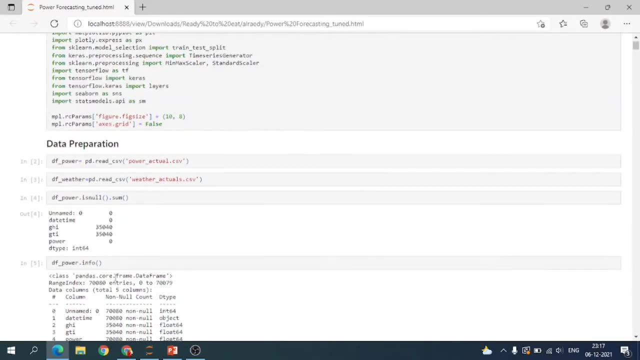 So the best strategy was to drop these columns altogether. Power generation of the PV model is noted every 15 minutes, so there are total 96 observations per day, And in weather-actuals dataset there were more than 13,000 entries with a time span. 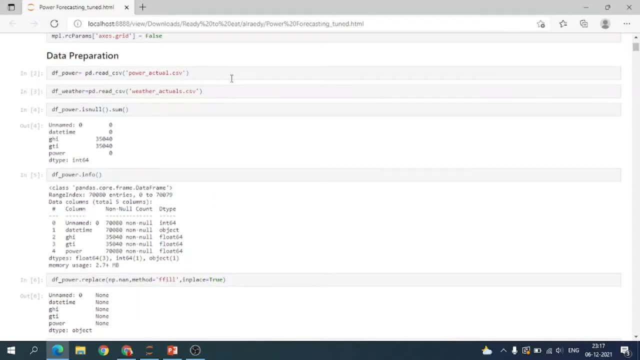 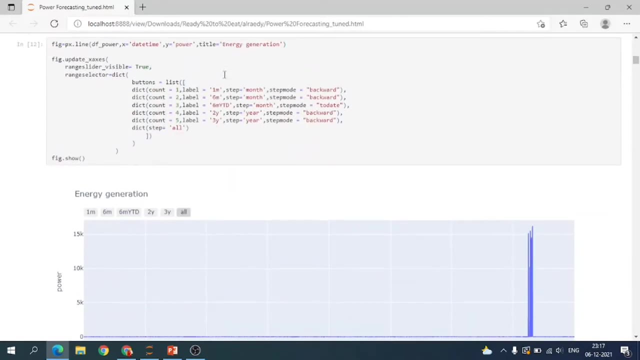 of 1 entry per hour, so there were 24 entries in a day. However, both the datasets were from the same period of time and hence I have used downsampling of the power data from minutes to hours. Also, the weather dataset was having some missing dates and thus I used forward filling. 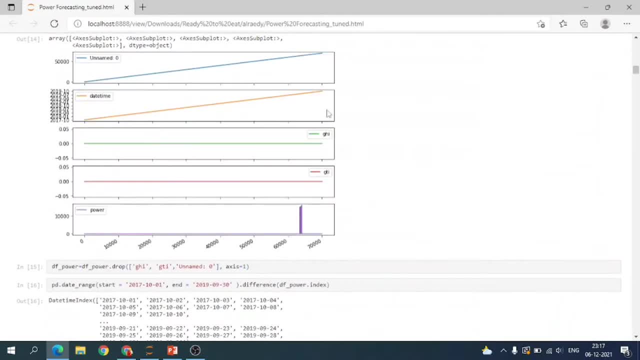 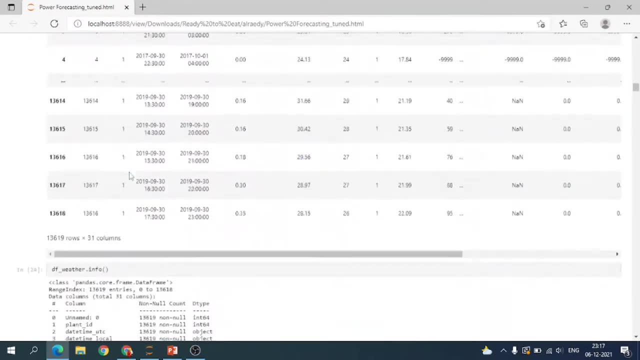 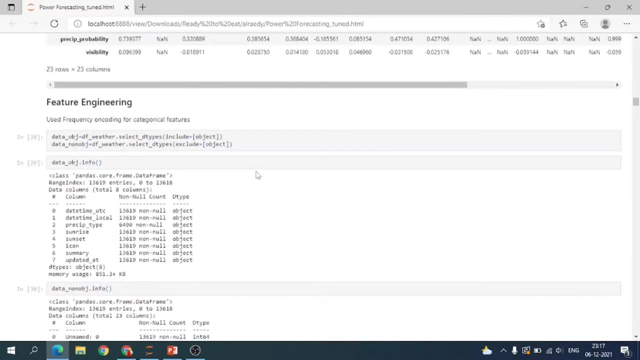 with mean method to impute. So basically, here we have dealt with the missing data and all, And then we come to the feature engineering. Firstly, I separated the weather data into object and non-object types so that it is easy to work with. 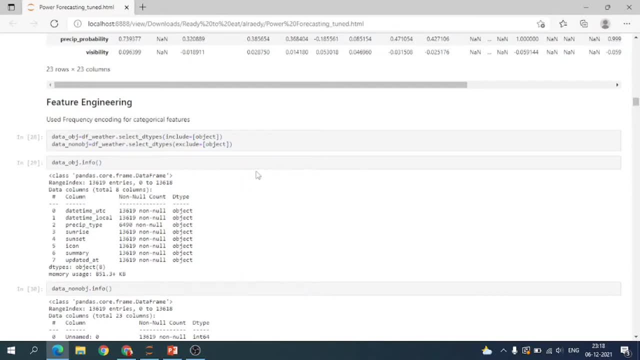 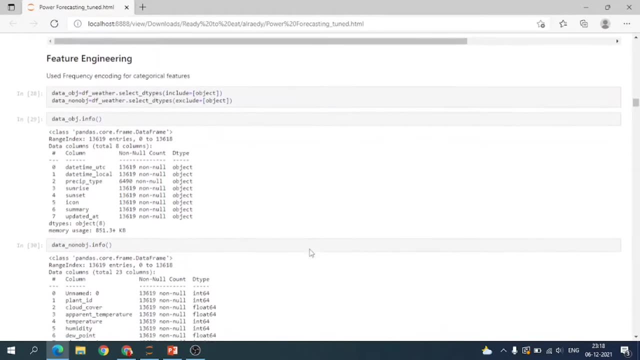 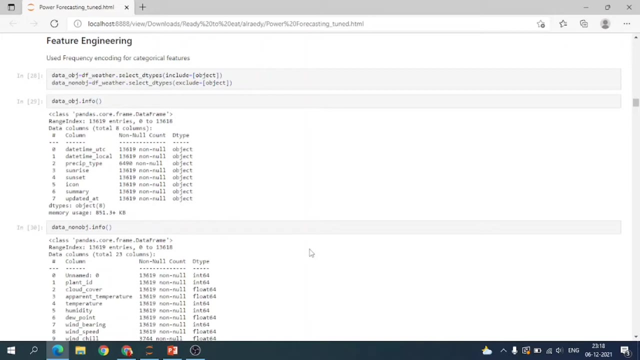 There were some features that we had to drop. I dropped initially- and most of them were duplicate data times and raw indexes For the categorical features in the object data. I used frequency coding to map the data points into a smaller and relevant scale After feature encoding. the graphs were useful for the purpose of finding out the category. 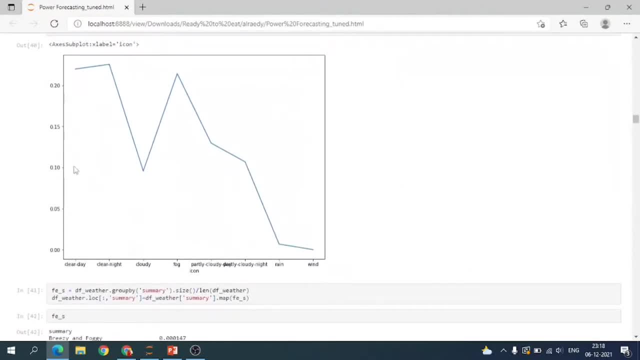 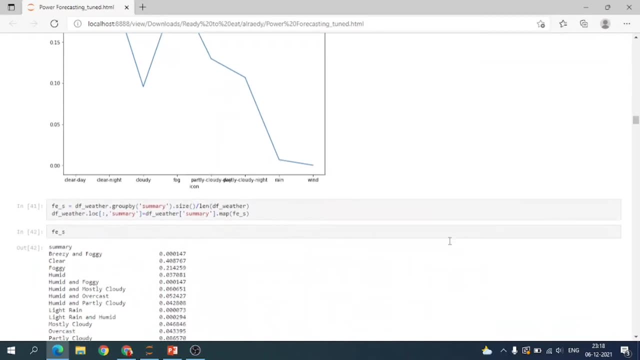 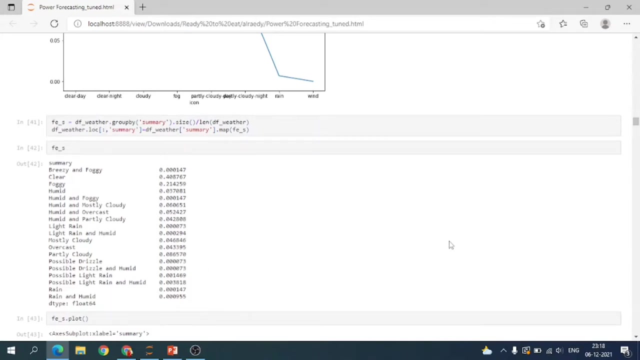 that was repeating the most in the dataset. So, from these plots, clear day was the most repeated category. There were some values in the dataset, For example weather dataset, which were given a value of minus 9999.. So these were nothing but the null values most probably produced by the IoT sensors. 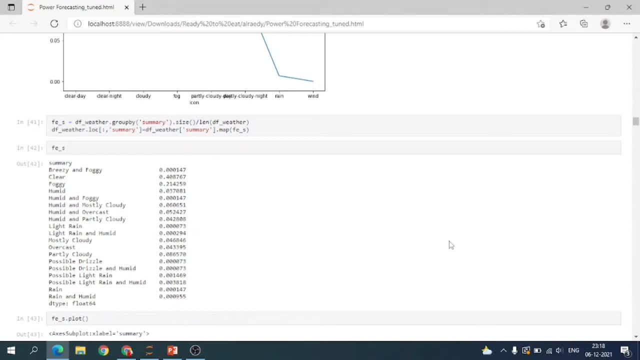 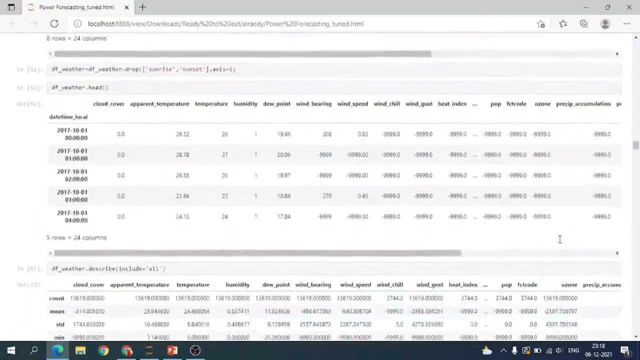 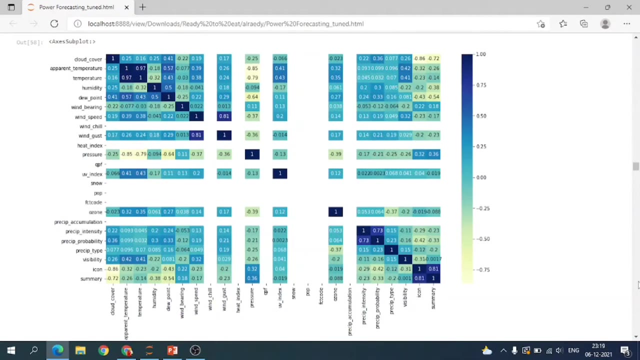 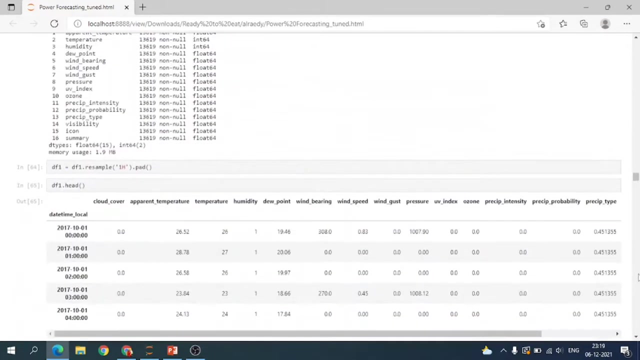 So these were also taken care in the code. After doing all this feature engineering, the correlation matrix- which will, yes, the correlation matrix showed us that only 17 features in all from the weather dataset were relevant. Also, after cleaning and looking at the correlation matrix, it was clear that there are very low. 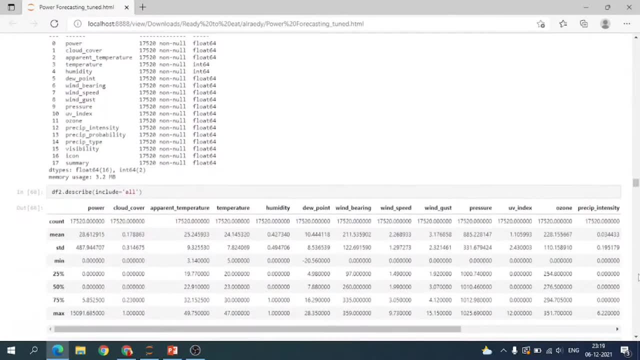 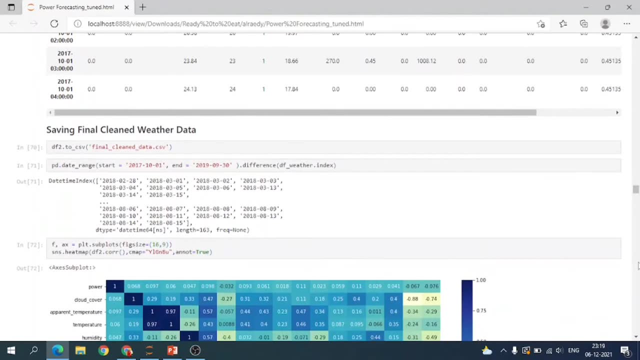 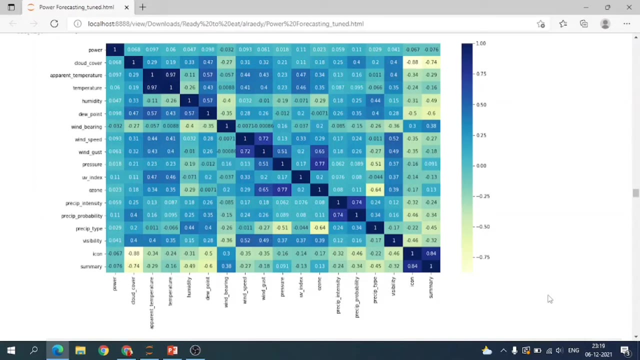 probability of snow and precipitation. at the plant site, There was very low snow and precipitation. That's why, finally, I drew a conclusion that the solar plant might be present in a desert type condition. So, basically, that's where we are generating how much power we will be getting from wind. 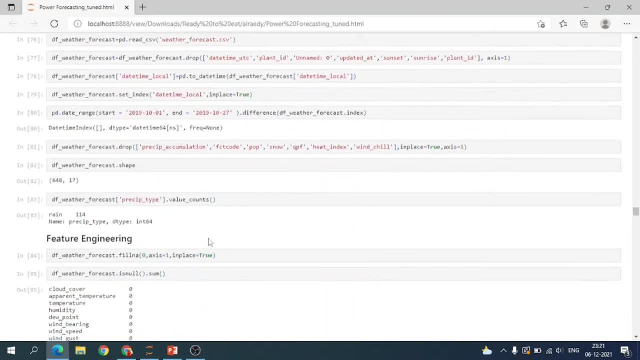 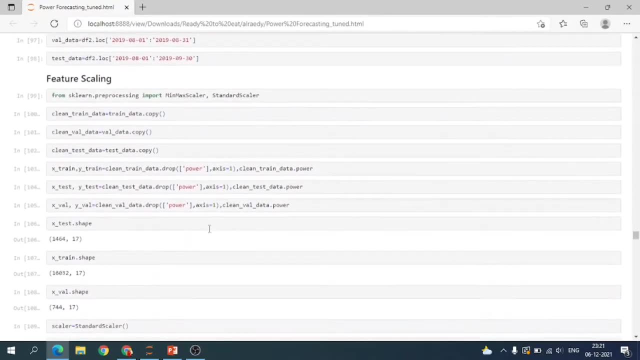 and solar. So yeah. So the next step which was done after feature engineering was feature scaling, So a standard scaler was used for scaling the data. As we know, it gives us a range from minus one to one. I would like to recall here that frequency encoding worked best in this scenario, because 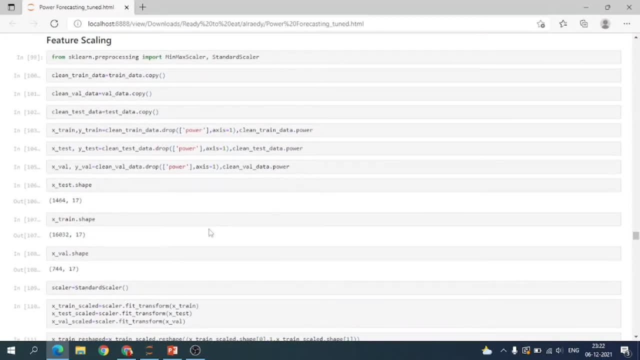 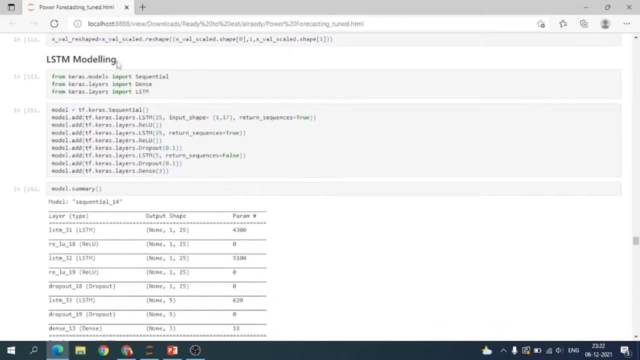 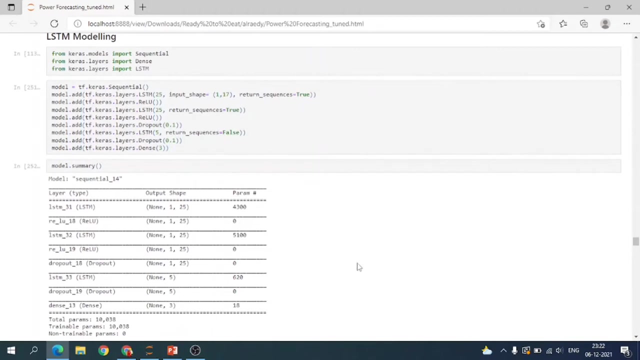 the features were not increased and hence dimensionally remained same, while reducing the range as well. Then we proceeded into the LSTM modeling, that is, long-short time memory. I have used slacked LSTM inside the RNN architecture for the purpose of building this neural network. 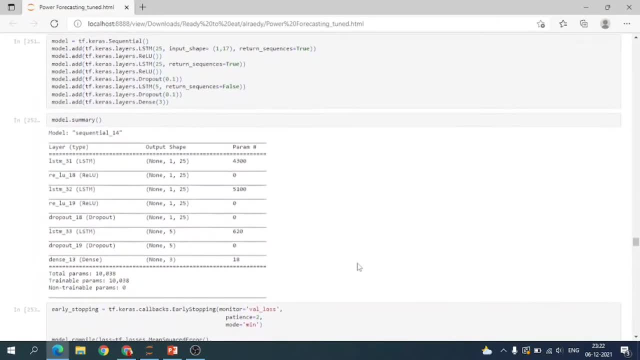 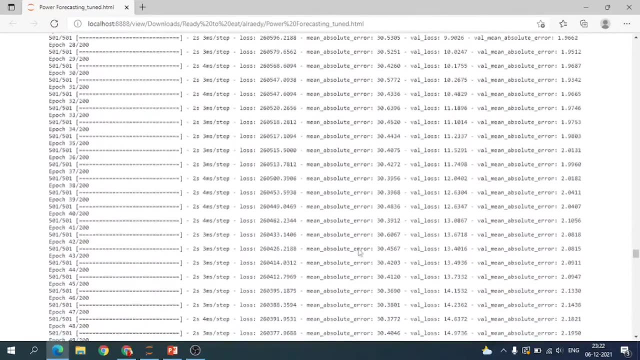 The activation function that I used was ReLU. Dense layers were also added in this architecture, So the initial model was having three stacked layers with 124 neurons for first two layers and then 64 for the third layer. So with the dense layer set to zero. 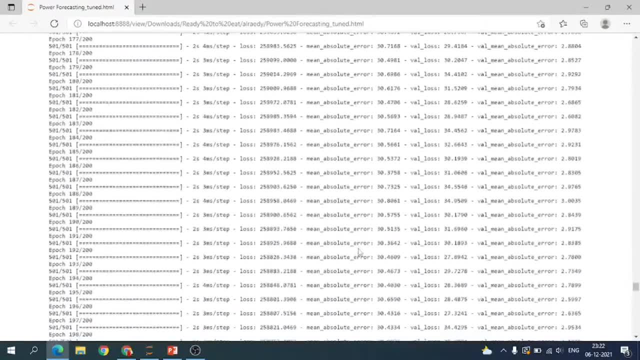 Then we proceeded into the LSTM modeling, that is, long-short time memory. So the initial model was having three stacked layers with 124 neurons for first two layers and then 64 for the third layer. So the initial model was having three stacked layers with 124 neurons for first two layers. 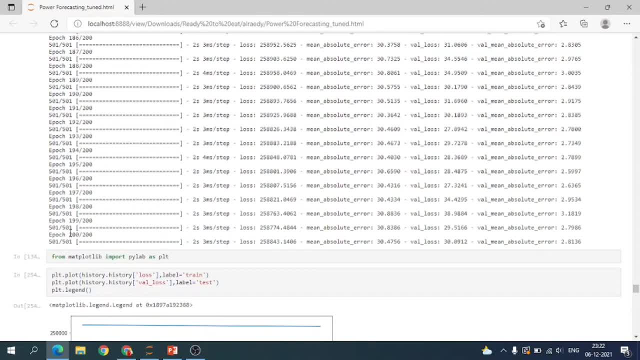 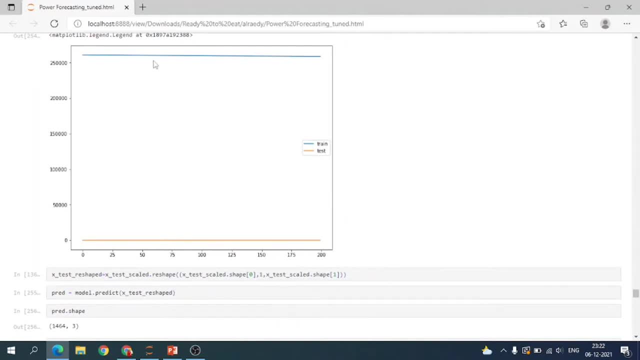 and then 64 for the third layer, So with the dense layer set to zero, And then we did a total of 200 epochs to reduce the error. And then, finally, we got a train test mapped and it showed us that it worked properly. 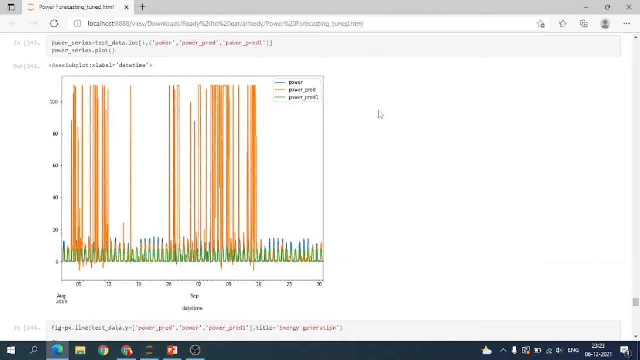 And after that- this was the final- three models were there. First was power, Then second one was named power prediction, And third one was power prediction And the third one was power prediction one. And from this plot we got to know that the power prediction one was the best model and 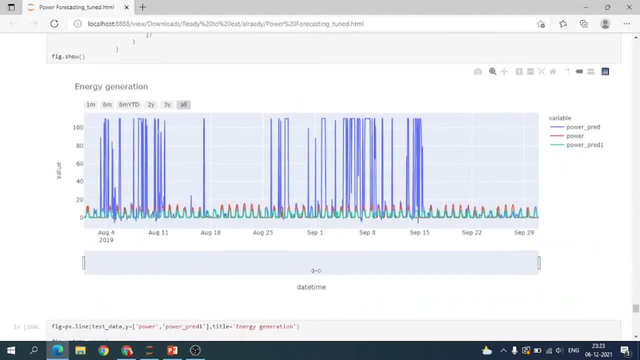 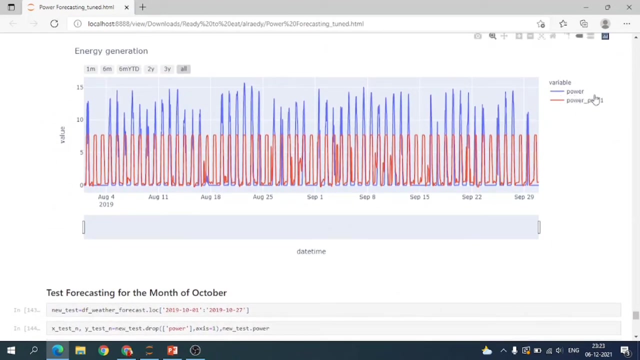 we took that. So if we see here this energy generation plot, we can clearly see that the power prediction one was giving us consistent output. So this was the best model and we have taken into consideration. So we have minimized it for the whole or we minimized into it into two. 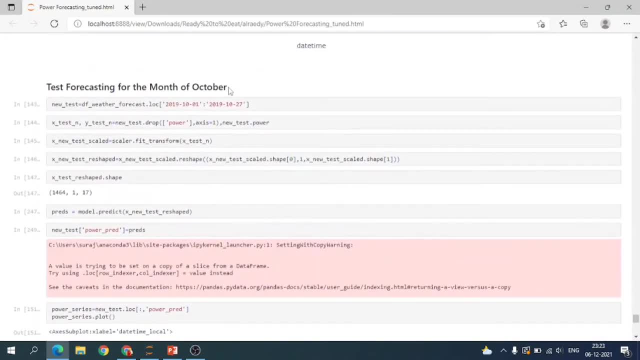 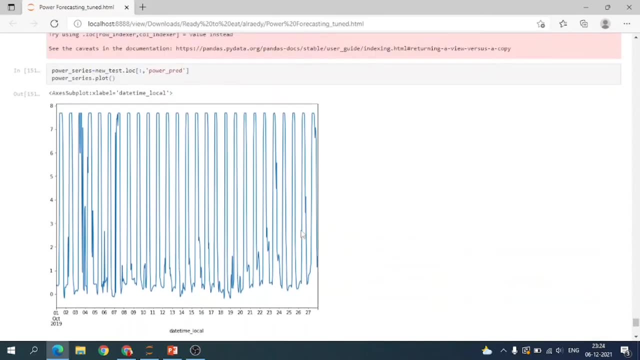 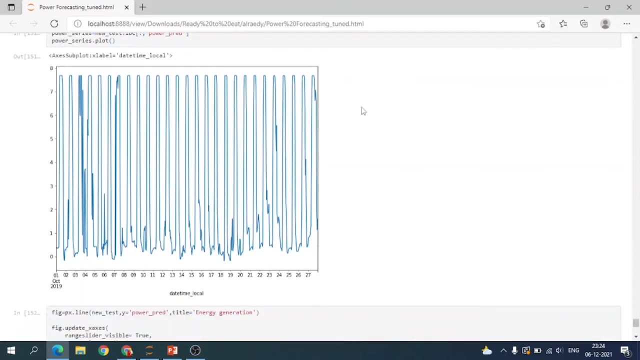 And then, finally, we did the testing for the month of October, which was initially to be done. All right, This is the power prediction, our final column that we have predicted. And after prediction, after predicting this, This is our, finally, energy generation.